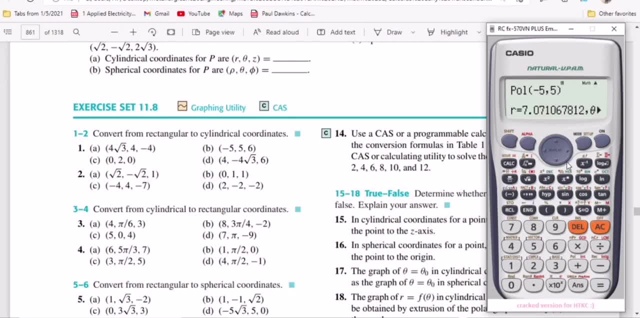 Equal to That means that R is 7 points, approximately 7.1.. And the theta value is- you shift here- It is 135 degree or centigrade, 135 centigrade. So but know that with the 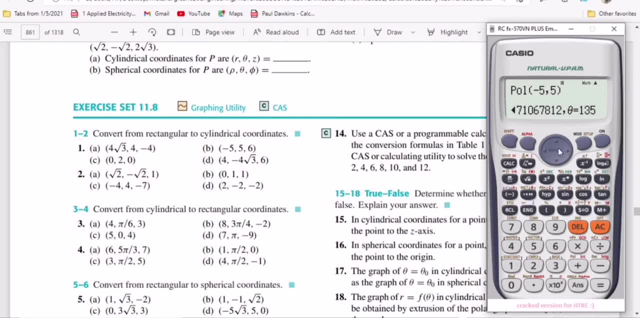 cylindrical coordinate Z is 6.. So with this, when you're expressing, you're going to express 7.1, comma, then 135 centigrade comma and 6.. Now let's go to the changing the cylindrical. 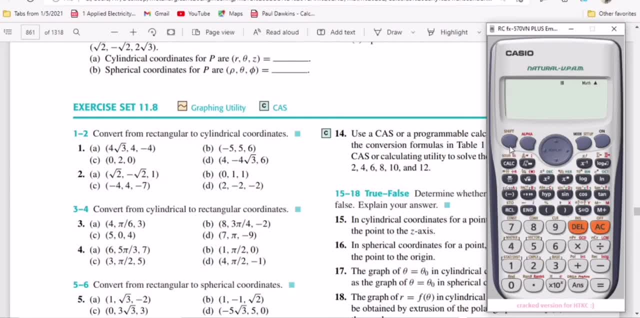 coordinate to the right. So let's go to the changing the cylindrical coordinate to the rectangular coordinate. What you do now is that you go to your calculator, you press shift and you go to: we have REC, REC. So then this one to apply for the same thing. 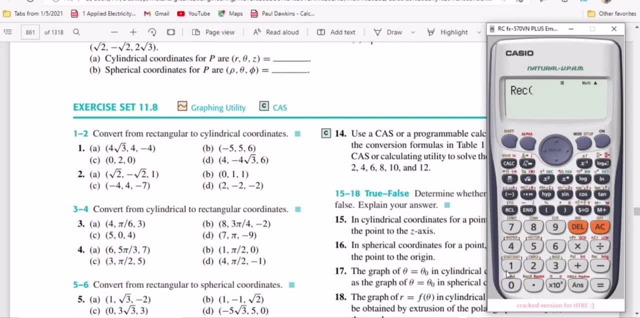 because Z is constant here. So we are not going to include Z, But we're going to include the R and the angle. So let's get going. So we have, let's choose. maybe let's choose A, So we put in 4. Then make sure you space out all. Yeah, You bring a comma, shift plus. 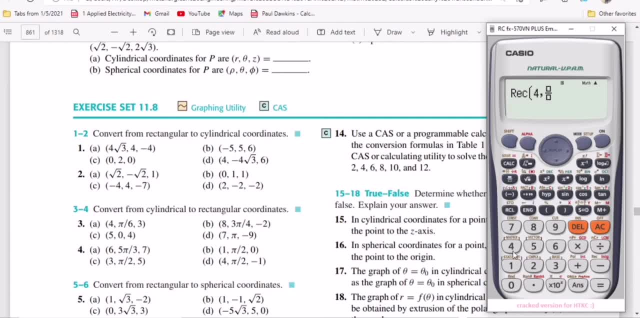 X, Then you comma, Then you bring this: Because pi is 180.. So 180.. Then you come down and you press 180 over 6.. You press 6.. Then you move here, Then you bring a comma, That's shift plus X. Okay, Sure, So with. 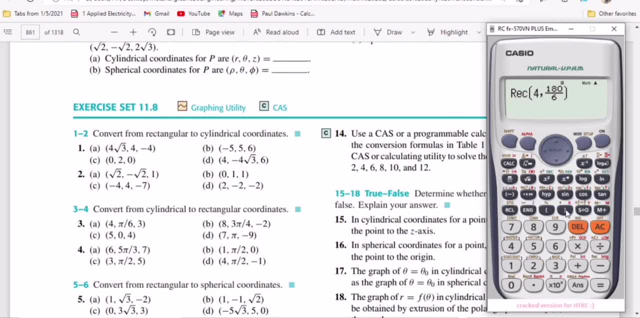 this. you're not going to include the Z, as the Z is constant. So then you press equal to. This is going to give you the X and Y coordinate. Then Z is constant. So we have our X to be 3.5.. So we have our X to be 3.5.. So we have our X to be 3.5.. So we have. 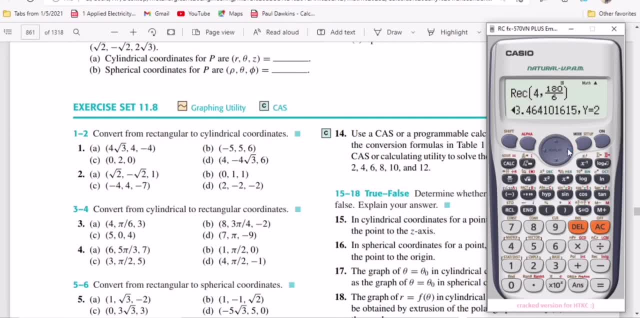 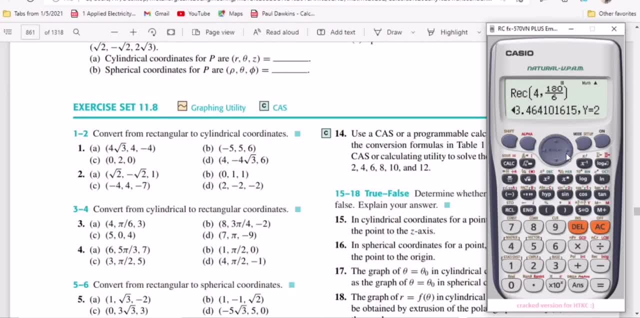 3.5, and the Y coordinate being 2. And the Z coordinate, you know it is constant, So it to be 3.. Very simple as that. Let's try another one and see. So let's go to shift plus rec and.